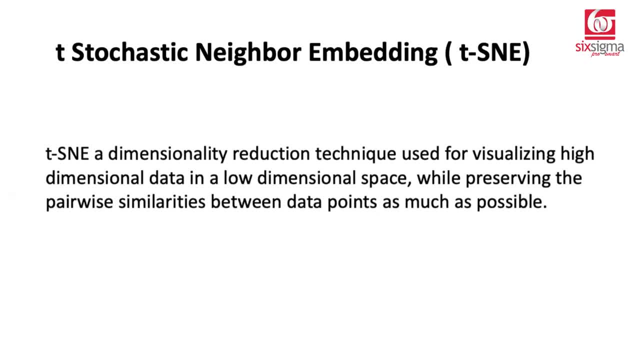 And trying to give you an output. It's not a transformation on the data, like PCA, which is coming up as an output that you can further work on. It is only going to be used for visualization purposes. Now let's understand. how do we apply this with the help of code, So we will go over. 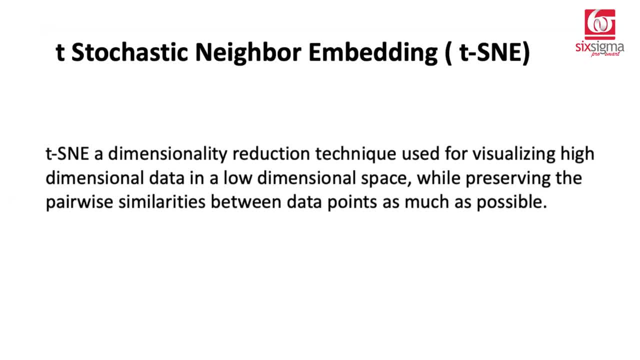 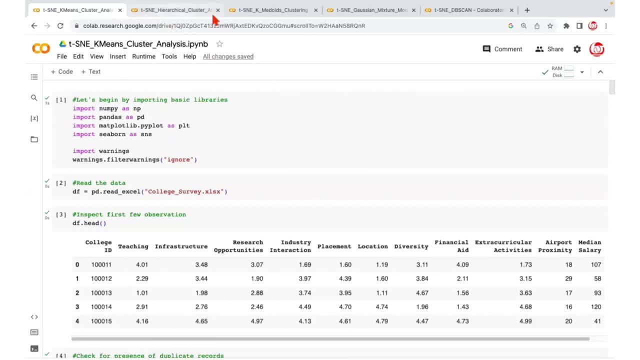 all the clustering techniques that we have learned so far and see how T-SNE helps us visualize them. Let's get started, All right. So I'm at Google Collaboratory right now and I've already opened multiple sessions so that I can just see what's going on, So I'm going to go ahead and open multiple sessions. 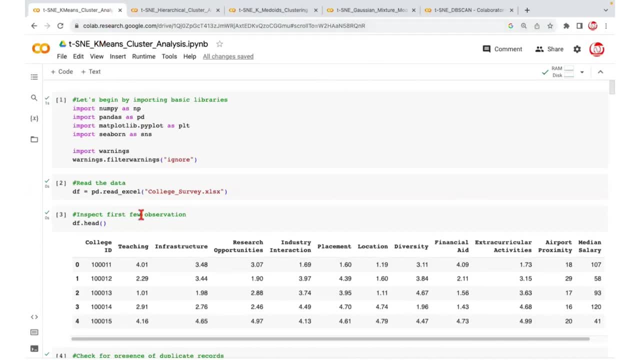 Let's get started, All right. So I'm going to go ahead and open multiple sessions so that I can just walk you through the step-by-step process. We will go through the complete step-by-step process for one type of clustering And for the rest it's just the similar execution, Just the labels are. 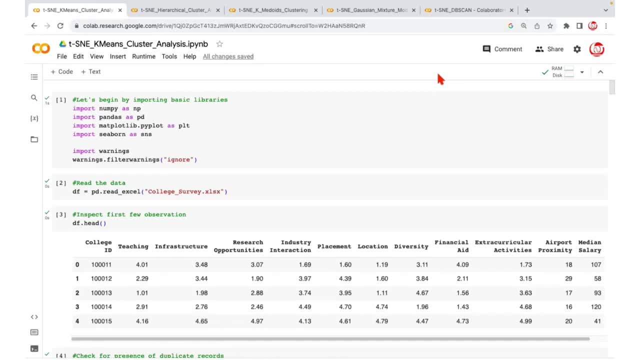 changing. For example, you are storing the labels to begin with as K-means, which later on becomes hierarchical, and then mid-wide, then Gaussian mixture and DB scan, so on and so forth. So we've been talking about this data right from the beginning, which is a college survey data. 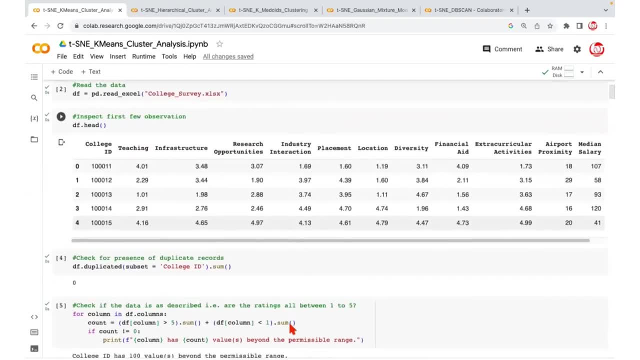 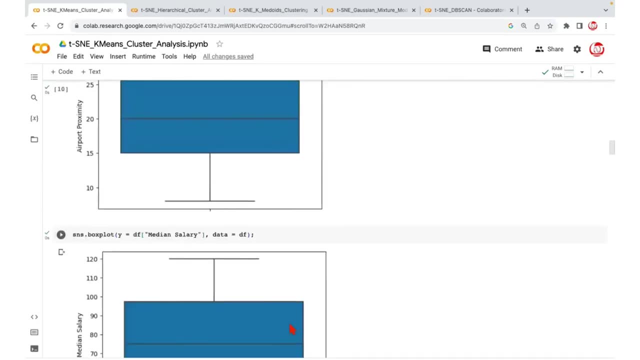 We've done the complete data preparation. Those steps stay intact. We're not going to change any of those steps for T-SNE. It's all going to stay the same. It's only once the clusters are achieved is when T-SNE comes into action. 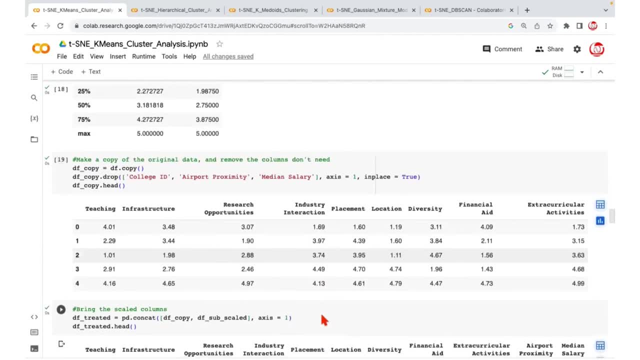 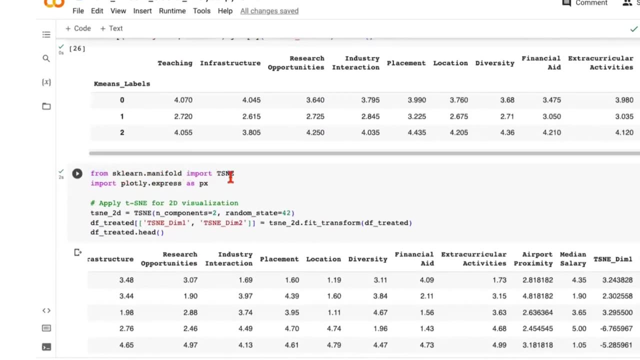 So if you've not followed the previous videos, you may want to follow the sequence of videos and you'll be then up to date. So T-SNE will take charge of the situation from this point on. What are we doing here? We are importing the T-SNE class from the scikit-learn many-fold. 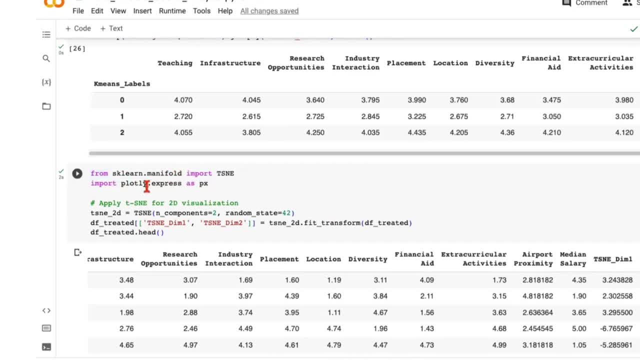 module and we are calling Plotly Express for visualization. This is a little better visualization, a little advanced visualization compared to Matplotlib and Seaborn, So we'd want to use this here. Just like we instantiate principal components, we can instantiate T-SNE. 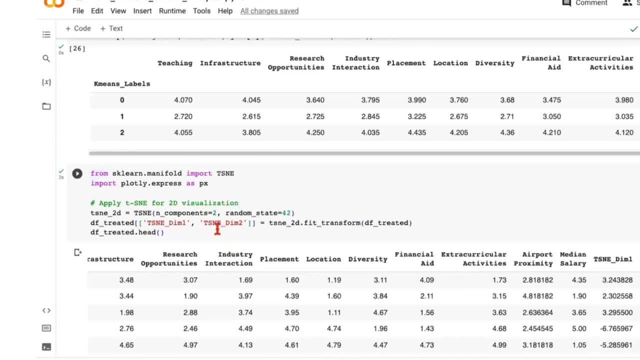 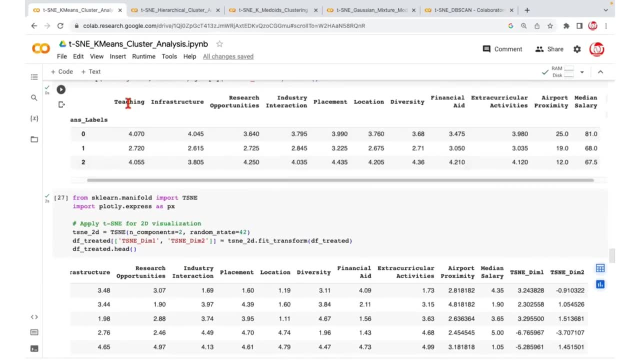 also, We have to mention a number of components. Now, number of components is basically going to be the number of dimensions to which the data will be reduced. If you realize, our data originally had multiple columns, so we had 11 columns to begin with, and we are saying that we want to. 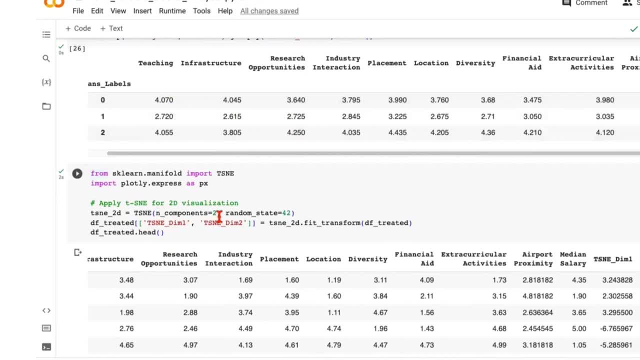 project this to only two dimensions to begin with, And later on we'll do to a 3D as well. We are mentioning a random state because T-SNE is stochastic in nature. As the name goes, stochastic means it's random in nature, So if you keep on repressing your code, 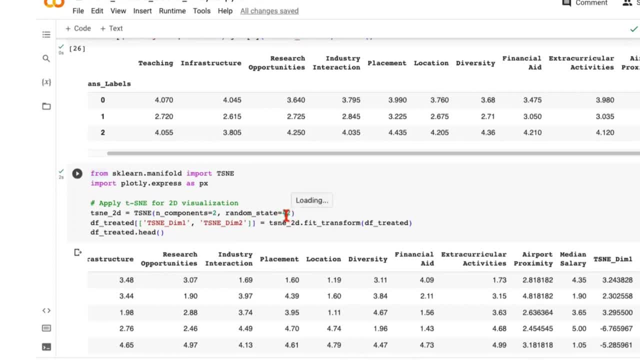 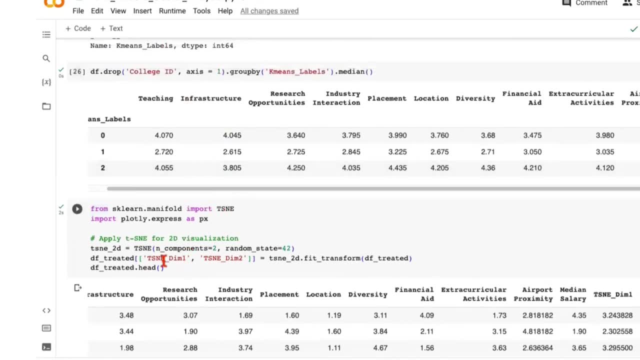 you may get different results. That's why this random state will ensure that our results are consistent. Now we are adding two new columns to our prepared data, not the original data, but the cleaned data, which we call as DFTreated. The first column would represent first dimension. 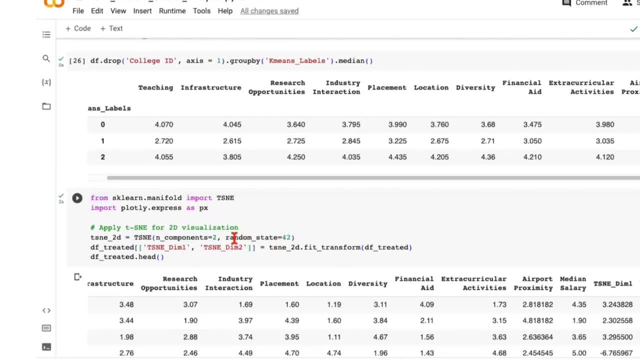 and the second column would represent the second dimension of T-SNE. Where would this come from? So if we do a fit transform on T-SNE is when we will get these two columns. If I show you the head of the data after executing this line, this is how it looks like We have two new columns added. 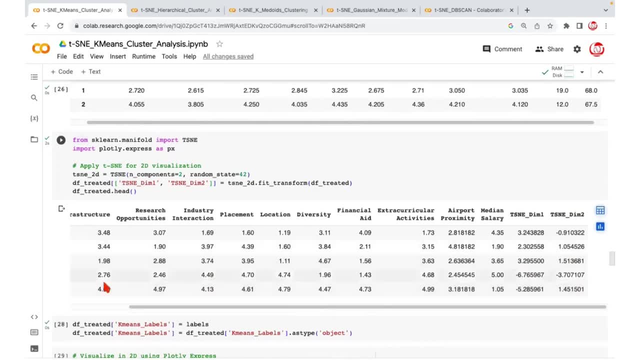 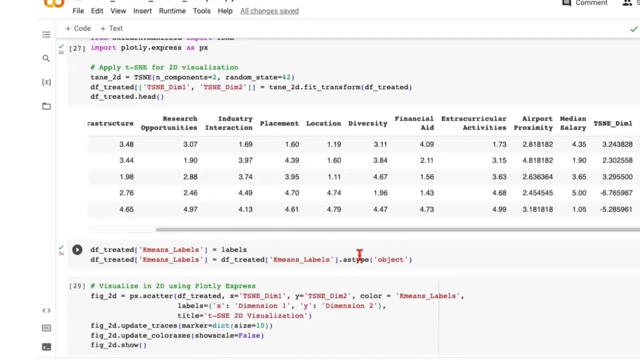 to our data. Now we are saying we will bring the labels to this data frame too and because we're going to be using these labels as the color or the hue, we have to convert it to the object type. Now this is a mandatory requirement for T-SNE, that if you want to bring the cluster labels as 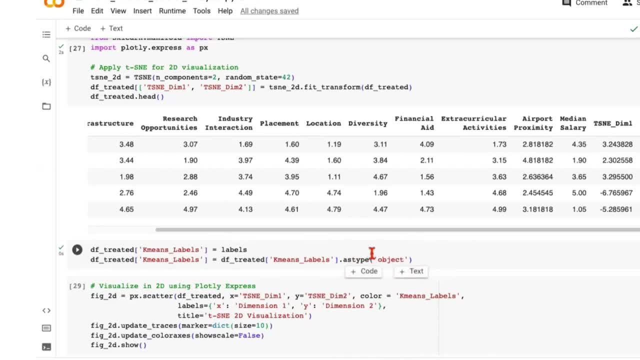 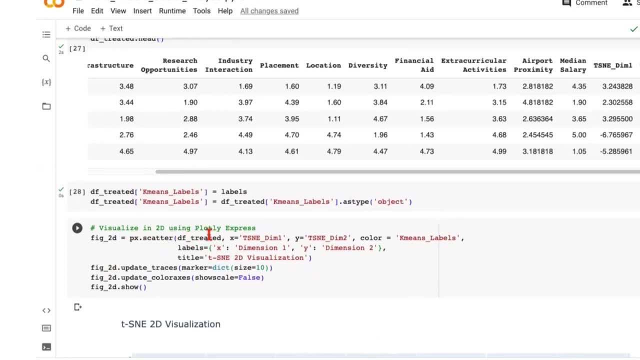 you have to bring them as string or objects. That's what we are doing here. And then we are using the scatter plot from Plotly Express. It's called scatter. We mentioned what do we want on the x-axis. It will be one of those reduced dimensions from T-SNE. 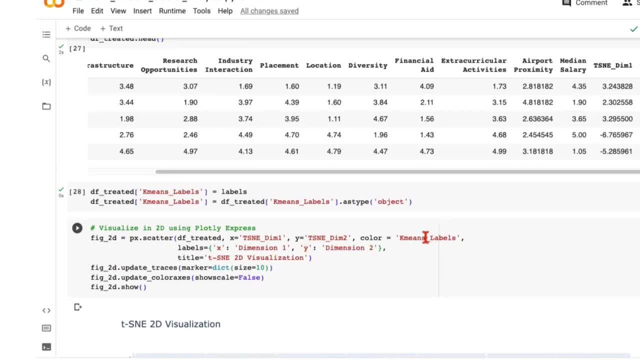 And y-axis would have the other dimension. The hue or the color would be as per the cluster labels. And then we are just mentioning the labels as we want to display on x and y-axis and a title for the plot. We are setting the marker size. 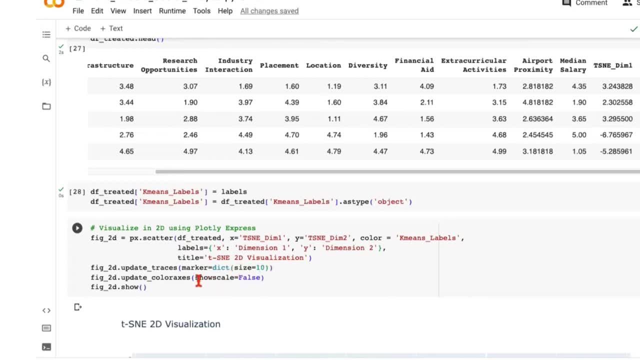 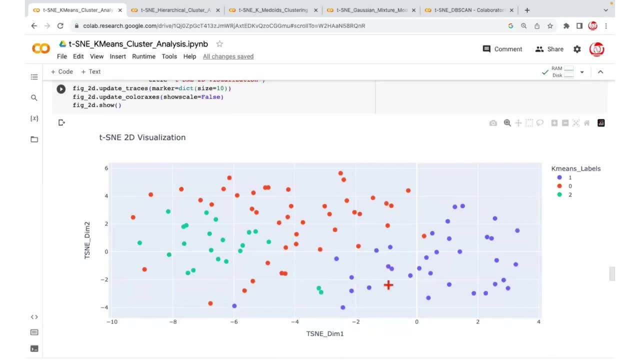 which is nothing but the size of the points that we will see, And we don't want any color bar, so we are just disabling that. Here is the outcome that you get Now, if you realize it has given a legend where it says: cluster 1 is here. 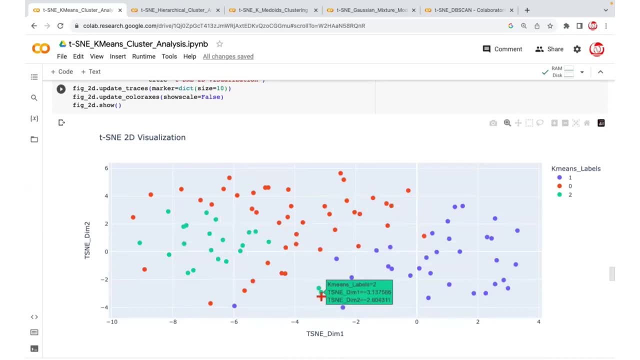 cluster 0 is somewhere in between and cluster 2 is here And there are some exceptions here. For example, some green dots you see here for cluster 2, some blue dots you see here for cluster 1.. There could be some exceptions. 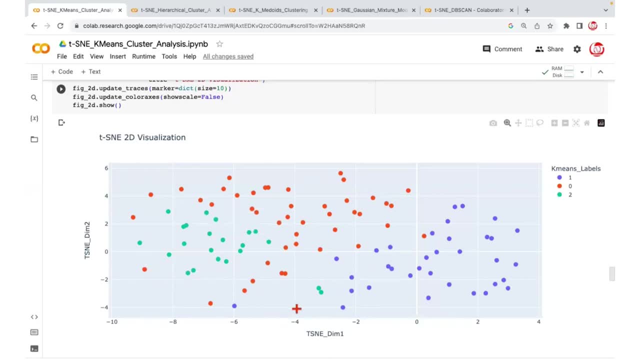 Remember all these techniques that we discussed. except for DBC, none of them was capable of handling outliers. So you may have extreme values which you will end up labeling something or the other, But it kind of suggests that between cluster 2 and cluster 1,. 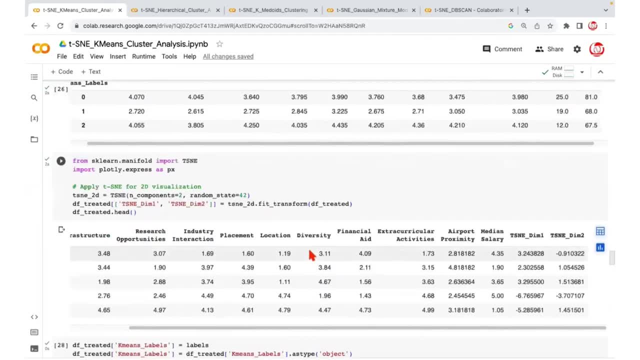 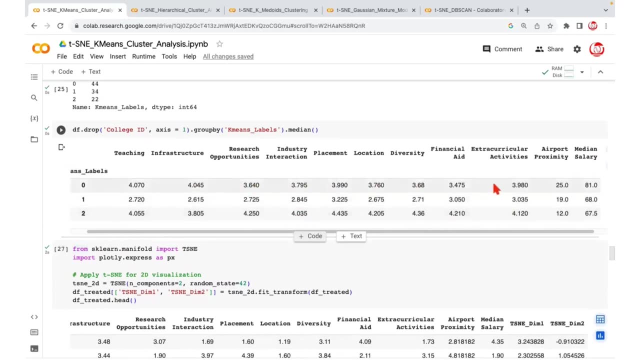 there would be cluster 0.. Let's see how our raw output was. So, if you see, cluster 2 were the best colleges, Cluster 0 were the second in terms of the ratings And cluster 1 were the colleges which were the worst. 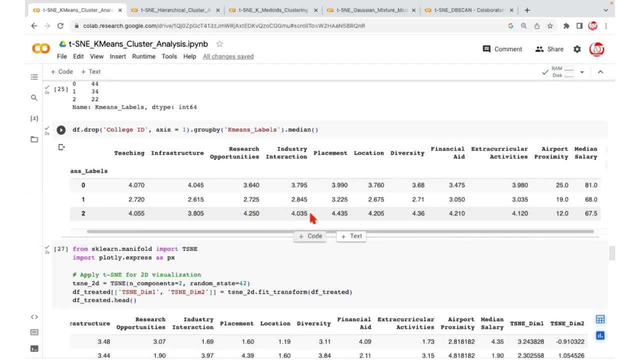 So ideally we should have cluster 2, on one side, cluster 1, on another side and cluster 0, somewhere in between, Because that's how we see it. in terms of ratings, Cluster 1 always had the most poor ratings. 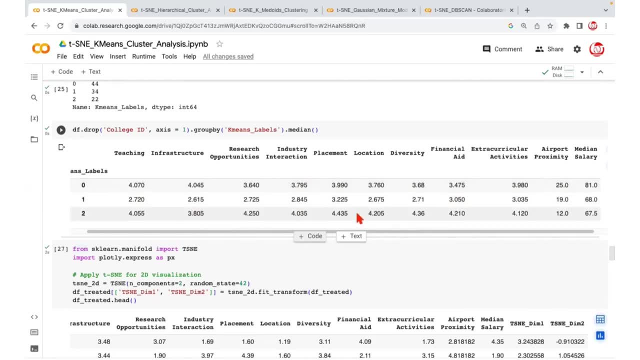 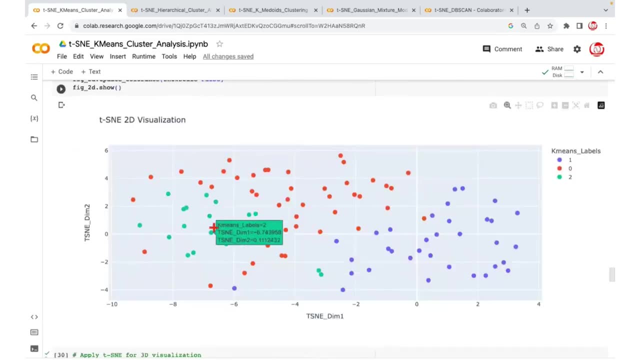 Cluster 2 had the best ratings. So between cluster 2 and cluster 1, there has to be a separation, And in between you will find cluster 0.. Is that how we see it here? See, so cluster 2 and cluster 1 are separated. 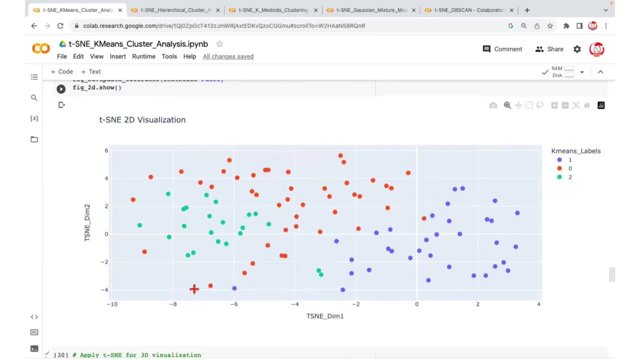 And in between we have cluster 0. Now there is no meaning of this x-axis as in. you might be wondering that you know. there is no meaning of this Cluster 2, if the best, it should be on the right. 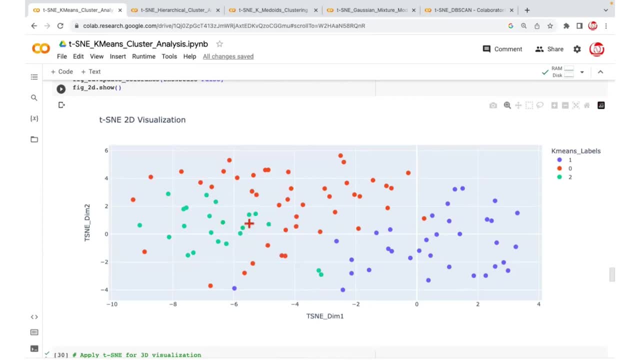 No, that's not how the axes are. This is a transformed space that we are looking at, So you should just look at the relative position, not in terms of scale or numbers. So we once again conclude that cluster 2 on one side. 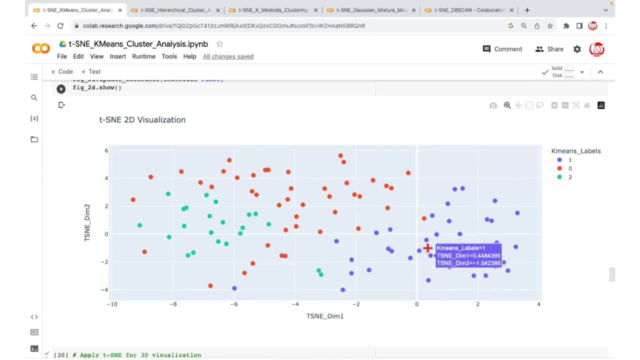 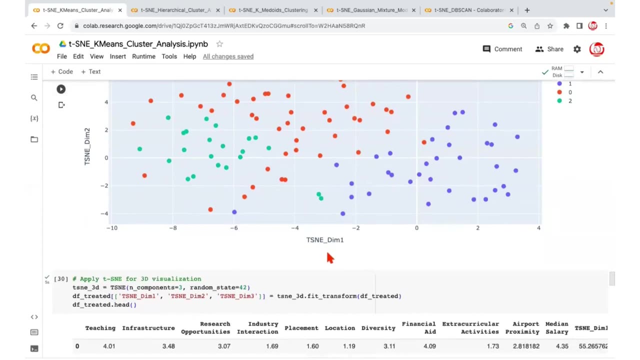 cluster 1 on another side and they have the maximum difference, And somewhere in between falls the cluster 0, right, If we were to look at it in 3D, it may be a little difficult to assess at first, but we'll have to exactly do same steps. 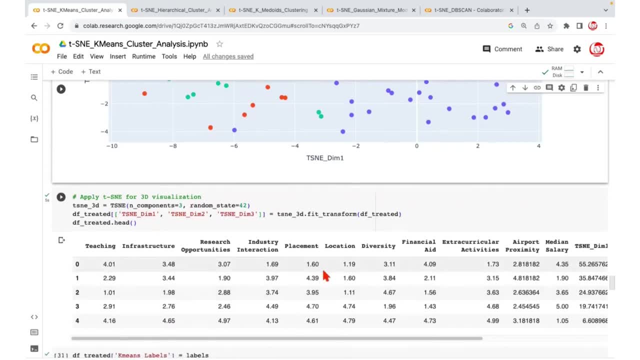 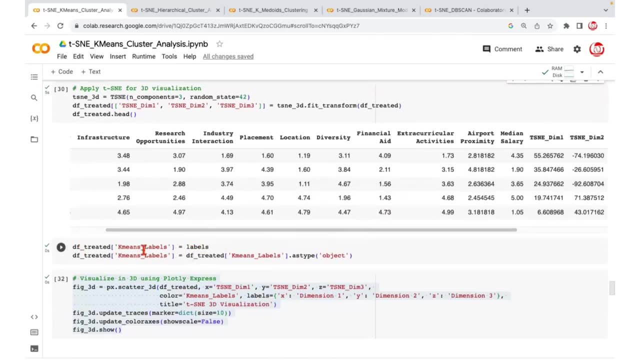 Well, we are once again going to give the number of competencies three and we are going to run this. It's going to give us three columns instead of two columns, because we'll be looking at these labels now and then we can add the cluster labels to this data frame as well. 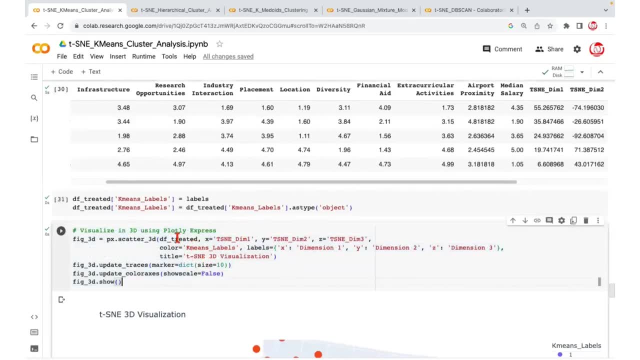 And then, finally, we can do a 3D visualization. There's not much of a change in terms of code, It's pretty much similar. It's just that in case of 3D, you also have to pass the third axis, which will be the third dimension in your data right. 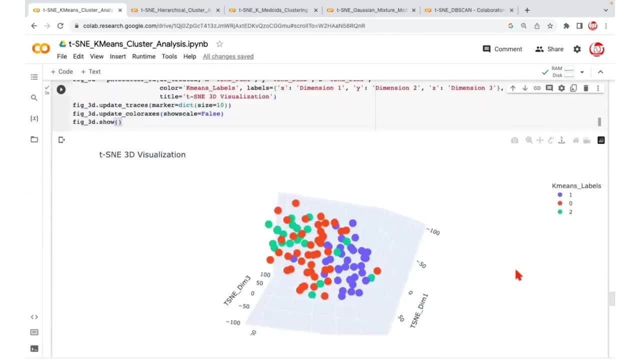 And if you look at the output, you will see something like this. You know, this looks a little complex to begin with, but let us see Now. do you get a sense that somewhere in this 3D green is on one side? 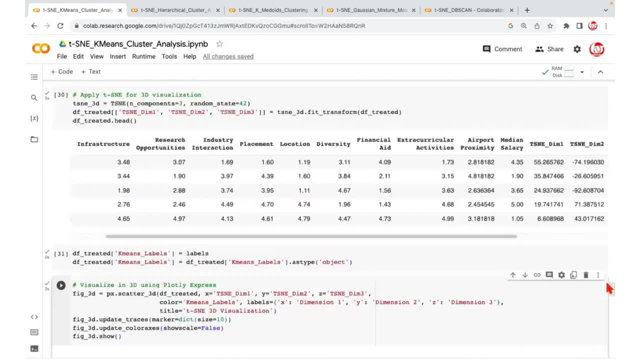 blue is on another side and red is somewhere in between, And if that is the case, then isn't it something that we saw here as well? right, So it's just a different angle from which we are looking at the 3D. 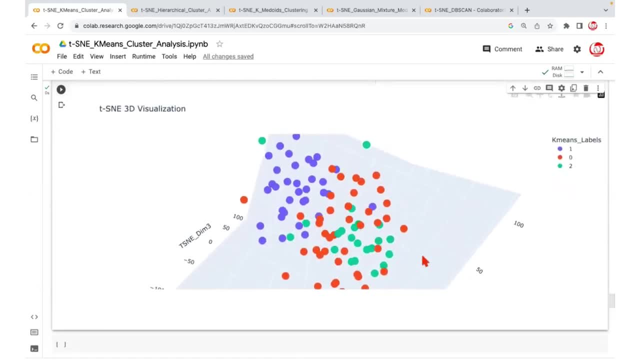 It's kind of conveying the same information. Of course, 3D becomes a little difficult to present and understand because it has a depth element too. If you kind of rotate it a little bit, you'll be able to see that you get an impression that. 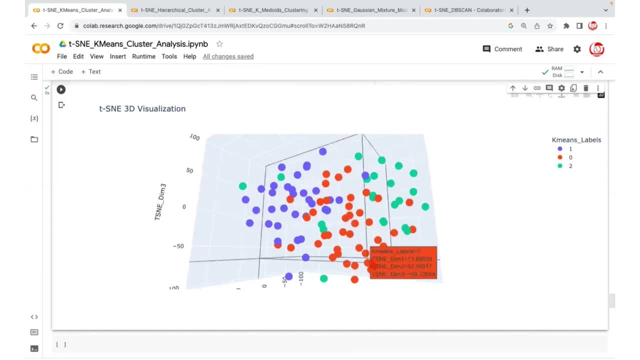 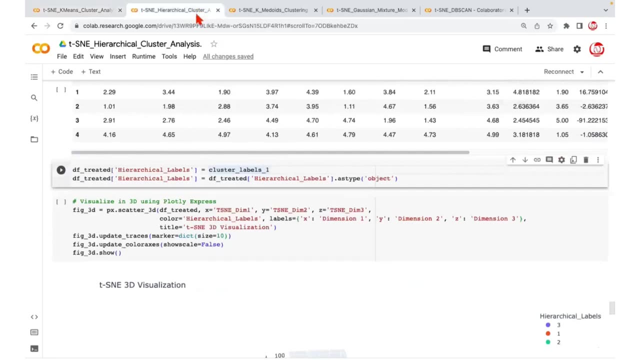 you know you have more of greens on one side, more of red in between and blues on another side right. So it's one and the same thing. Let's just see the output for hierarchical clustering. It's the exact same process that we have followed. 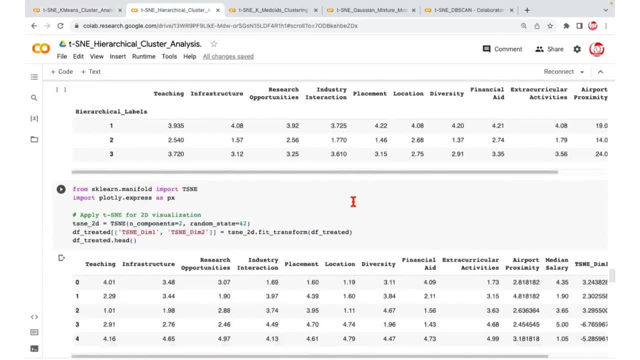 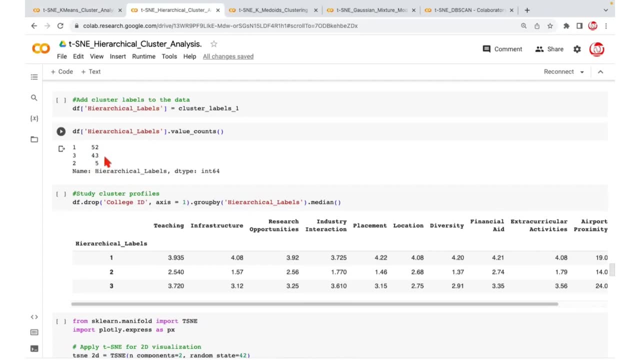 And we are going to look at D2D. Now, if you see, hierarchical clustering labels that we got were imbalanced. for a class two it was only five colleges that were given this particular class and remaining two clusters were kind of compatible right. 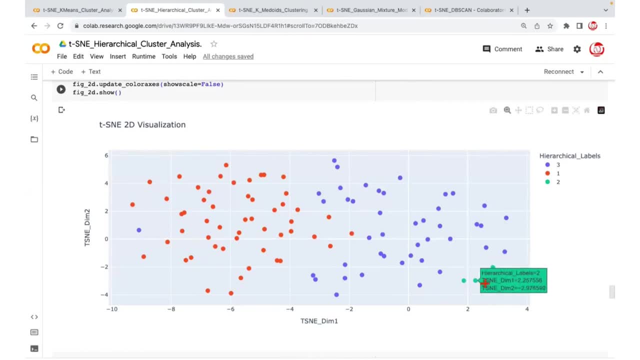 So if we come back to this, you can see that these are the pipe labels here for for colleges given to cluster two. then you have this blue and this in red, And there could be, of course, such cases, like you know. 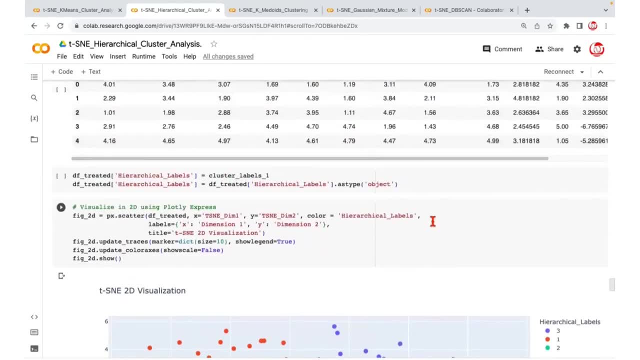 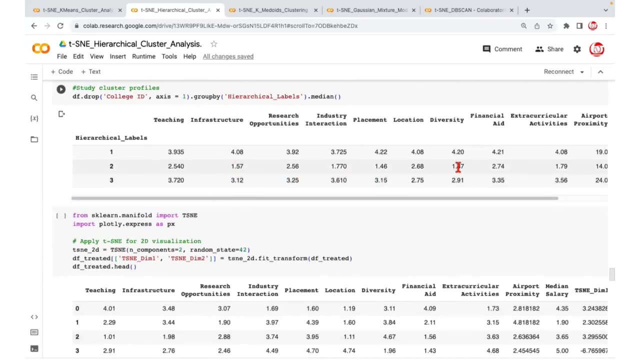 extreme values, which are given one or the other label for sure. So let's understand this here. in this case again, class two or the label two was the one which was the lagging most, label one was the best and label three was somewhere in between. 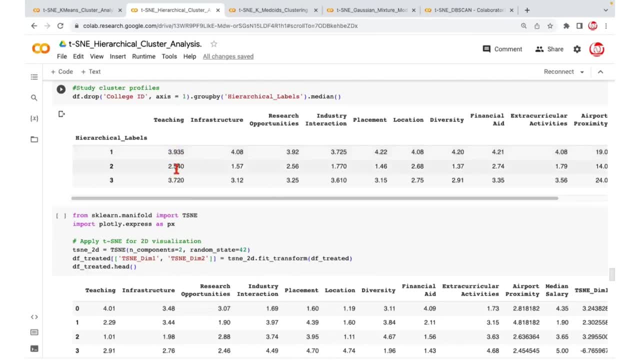 So the one should be on one side, two should be on another side And three should be somewhere in between, because this has values in the middle, not as high as one and not as low as two. Is that how we getting it right? 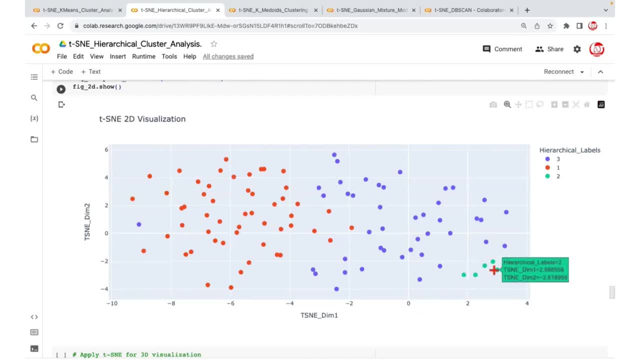 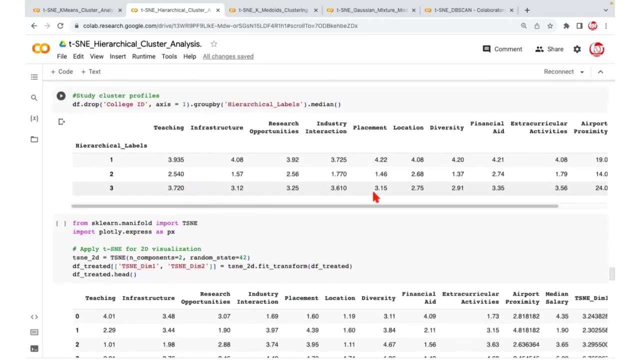 So, if you see, it's one and the same thing. so you have cluster two on one side, cluster one on the side and three is somewhere in between, just like here, three is somewhere in between. That's how it's supposed to be in terms of that. 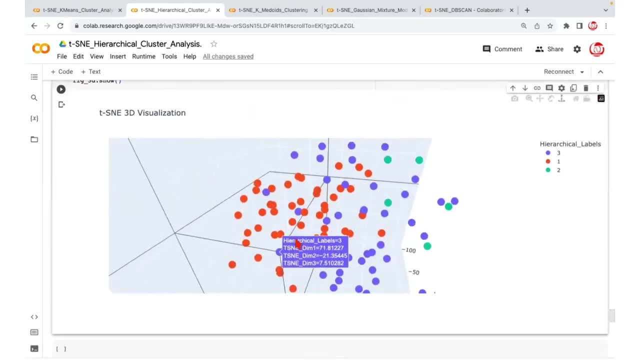 And, once again, if you look at this in a multidimensional space, of course, zoom in and you can see that these are the five points here And here also, you get an idea that- and of course there are places where blue and green are kind of overlapping. 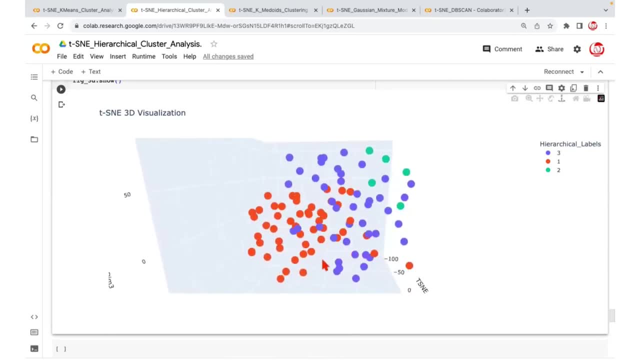 but red is largely on one side and it's separated from green, and blue is somewhere in between. So again, the logic of clustering was different. It is able to cluster, but the labels could differ, and this is unsupervised learning. So there's nothing right or wrong. 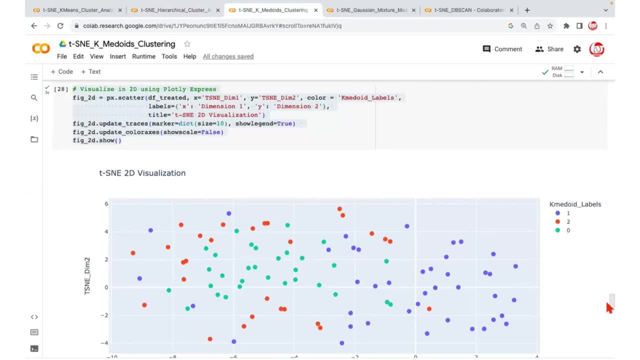 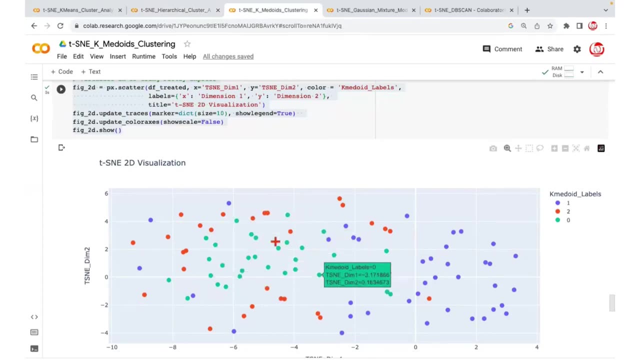 You're just exploring the patterns in the data. Then we also discussed the Medoids clustering, and this is how the output from a Medoids- right, So Medoids, if you see- is a little different in terms of shape. it's kind of that green is being enveloped by the red points. 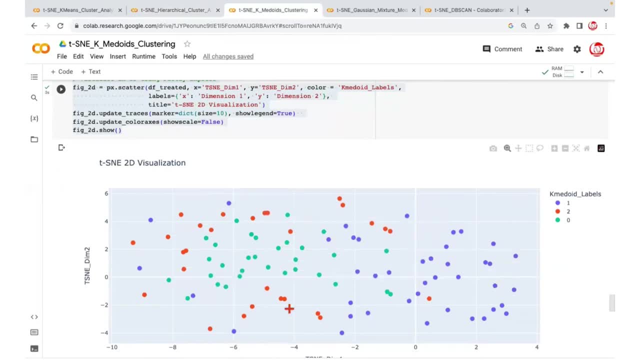 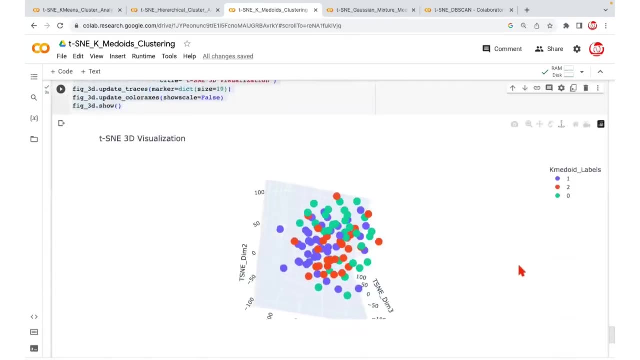 here. Blue is on one side, green is on another side, but green is kind of envelope by the red points here. That's how we get the out. If I show you the 3d visualization for Medoids, it looks like this again: 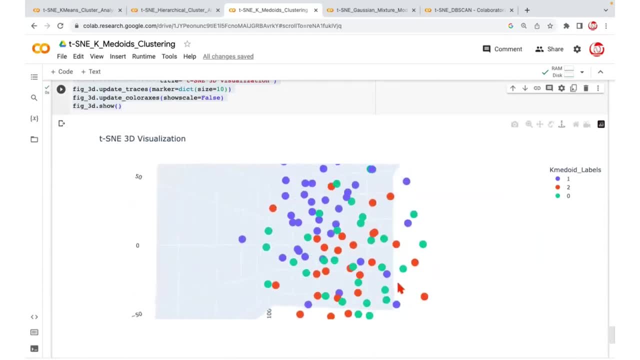 So do you get an impression that green and red are kind of mixed up and blue is on another side? largely, see, blue is kind of separated. Red is coming to the front here and also located at the back, So green is somewhere in between. blue is on one side. 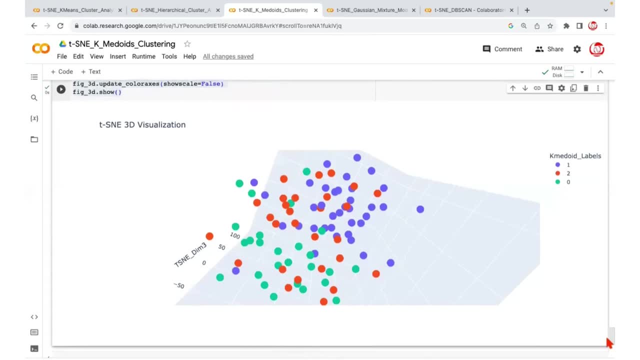 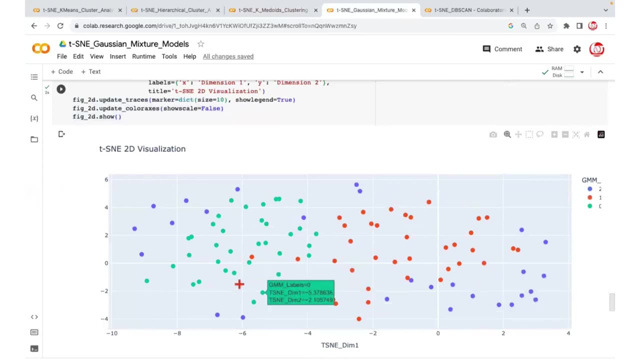 and red is enveloping the green. That's the kind of impression you get here. Okay, Let's look at the same thing: the Gaussian mixture model. So when we come to the Gaussian mixture models again, you can see that Gaussian mixture model was a soft clustering. 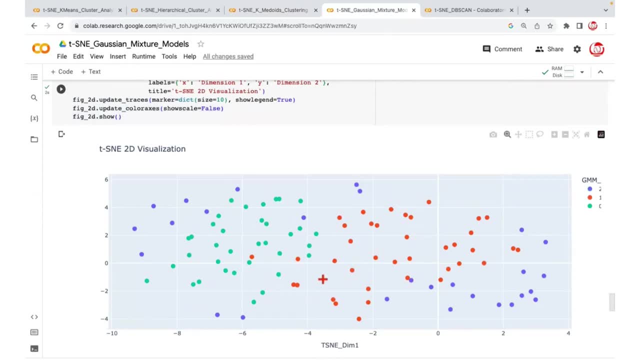 technique right. So it will be totally flexible, with the points kind of overlapping here and there And you can see that there are some blue points here and some blue points here, green points in between and red points in between. So Gaussian mixture model was a very flexible approach to clustering. 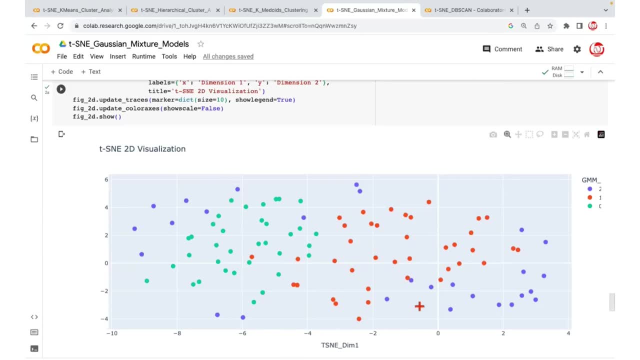 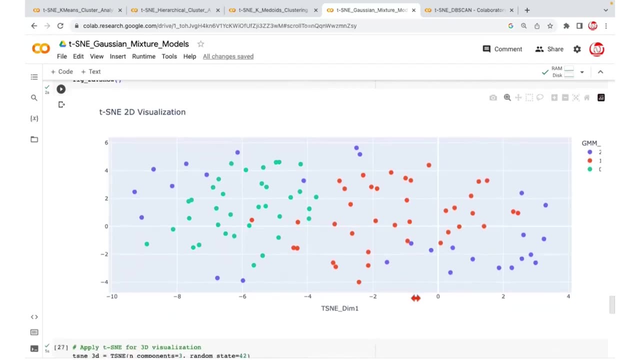 And that's why you could see a mix of points everywhere. Once again, remember Gaussian. mixture models too, are sensitive to outliers, right? So when you have outliers, they'll be given some of the other labels for sure, And it may not be the best label. 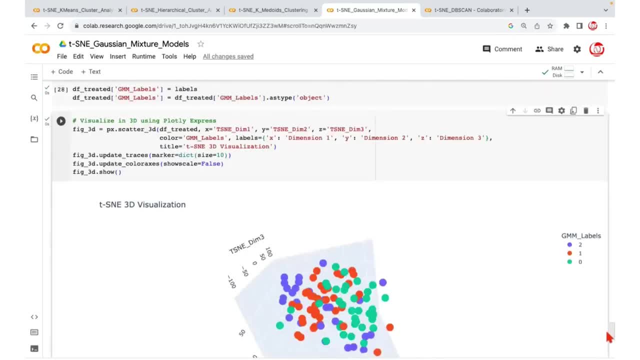 right. So you could have such exceptions here. And if you look at the 3d, I'll just scroll down a little bit. If you look at the 3d here, what do we see? So we see a lot of mix here. 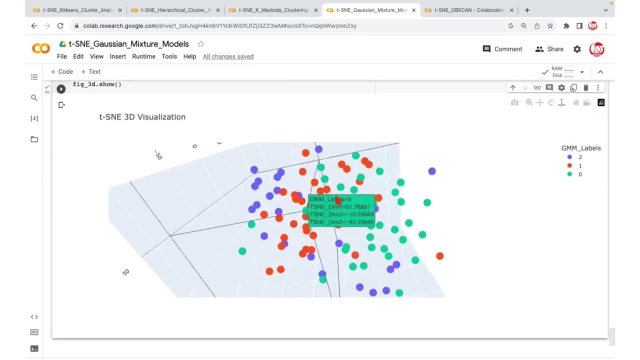 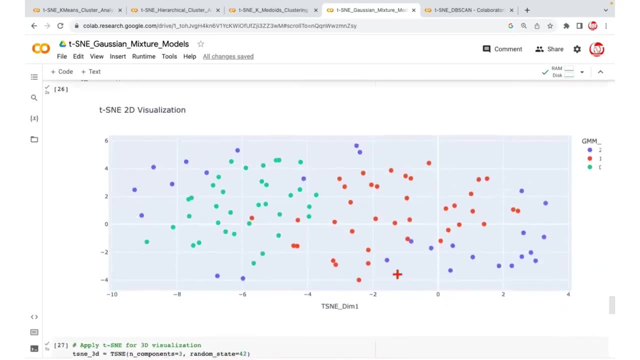 right. So you can see blue is here, Blue is here as well, Green is here and green is somewhere here as well And red is somewhere in between. So you kind of get the same impression right. So it's it's more spread out kind of clusters that you see so far with the conventional 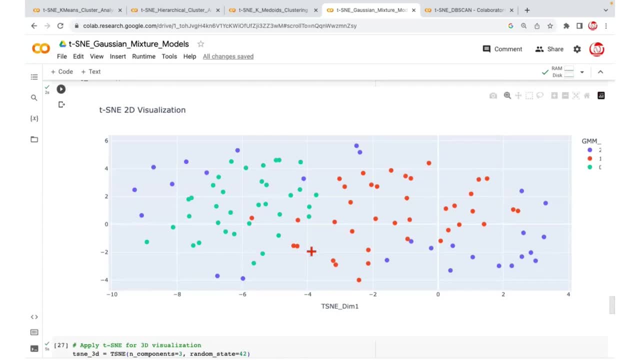 right, So it's. so. it's more spread out kind of clusters that you see so far with the conventional techniques like means, midwides and hierarchical, We were getting a very nice separation. but there could be such data sets where a mix actually makes sense. 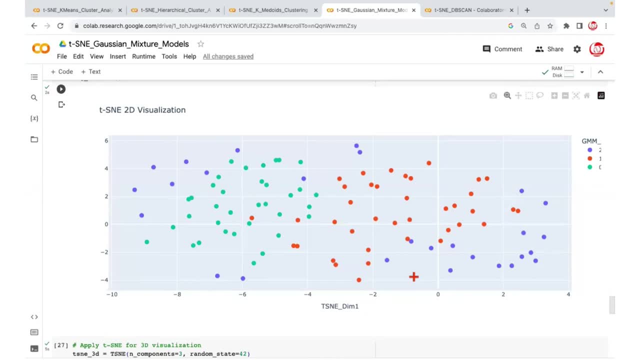 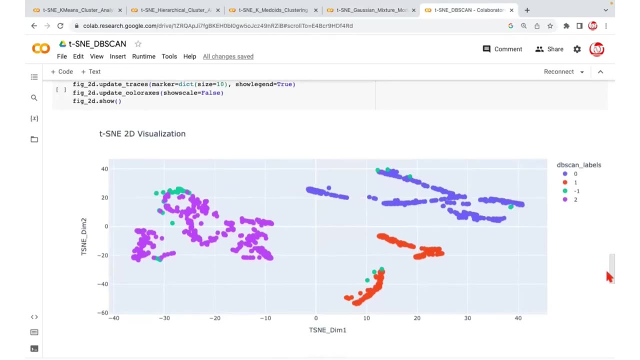 You know, this point could still belong to the red cluster because of the red Gaussian, And that's what this proves. So the style is very different. Now, finally, we come to dbScan. but dbScan is something we did on a different data set. 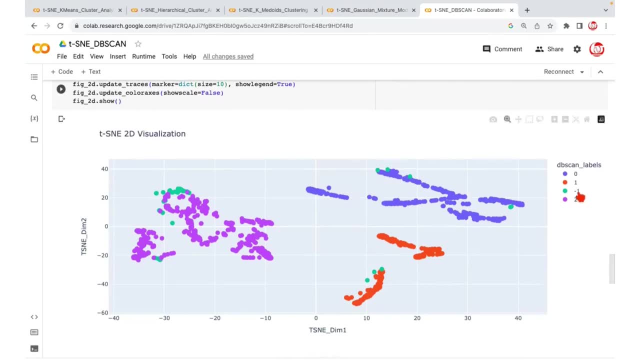 right And dbScan was smart enough to be able to point out the outliers with a minus one category And you can see there are some dots here which have been pointed out as outliers. So we discussed the concept of core points, the boundary points and the outliers. 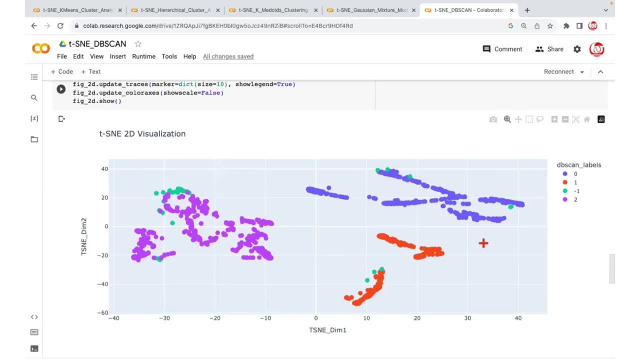 right. So core points of course, joined the clusters, their boundary points or the neighbors also joined the clusters, but outliers are segregated And this is what is happening in this particular case, If you recollect the kind of distribution we got. 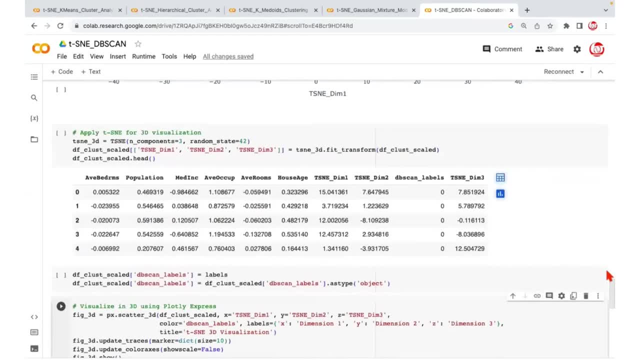 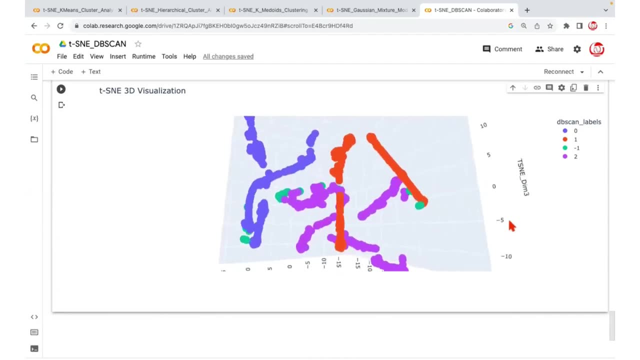 we had about 52 outliers and this is how the labels work. So if you look at the 3d representation of the same, this data set is different, right? So you can see this forming clusters in a very, very different way. 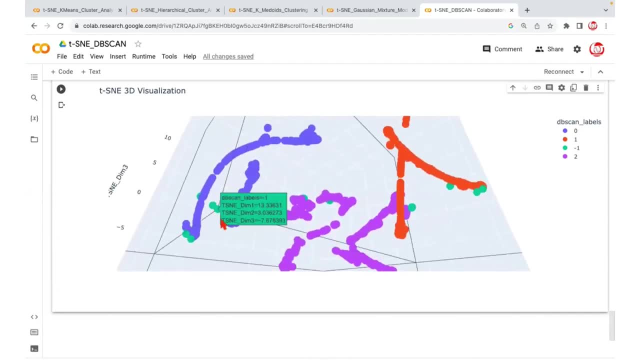 And it's pointing out outliers. Now you may not be able to visualize and say that why is this point an outlier? Because, see, if you, if you look at it like this, it looks like green and blue are all overlapping, but the moment you zoom in, 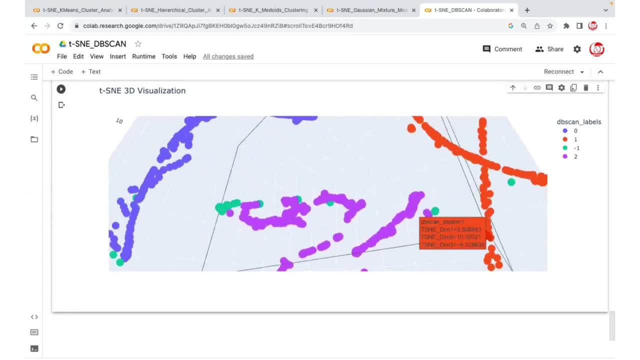 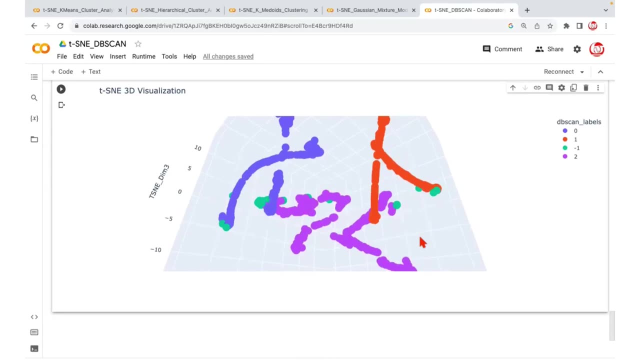 you realize that there's actually a difference, right? So 3d could be a bit confusing to begin with, but you know it has worked on the same logic that we discussed in our theory videos earlier, right? So this is a very powerful technique when you have to visualize. 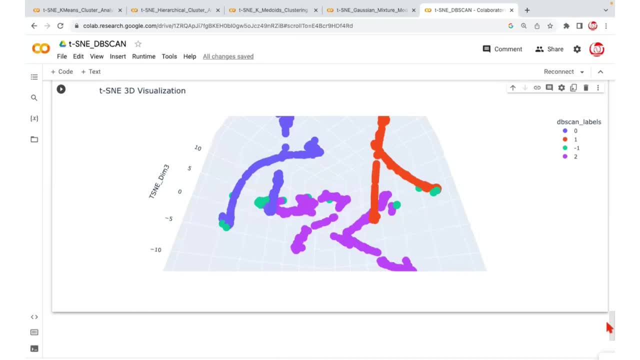 the data which comes in multiple dimensions- In our case it was as high as 11 dimensions And some of the data sets. but it has been able to nicely give us an impression on 2d and 3d, 3d with a bit of effort to analyze.